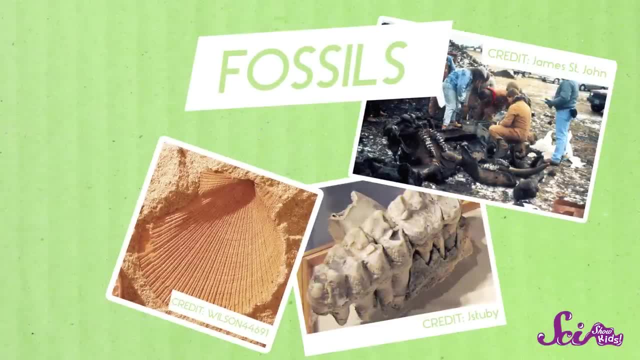 Fossils can be of animals' bones, teeth and shells or the imprints of old leaves, Or they can be rocks that hold other clues to what life was like in the past, Or they can be rocks that hold other clues to what life was like in the past. 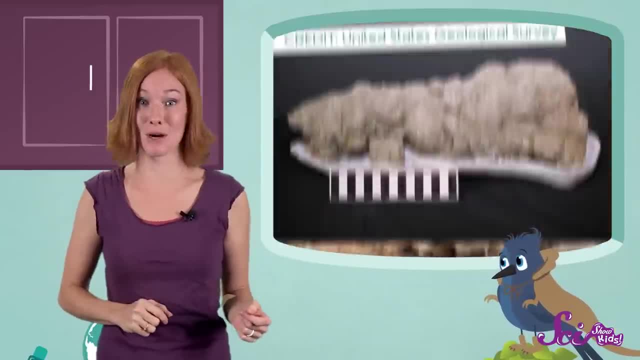 Or they can be rocks that hold other clues to what life was like in the past. in the past, like an animal's footprint or even their fossilized poop. Paleontologists use all of these kinds of fossils to find out more about the history. 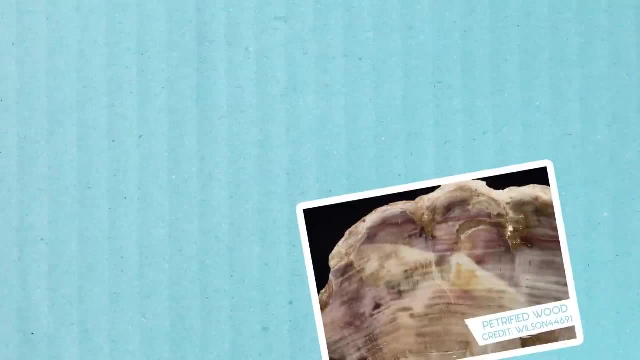 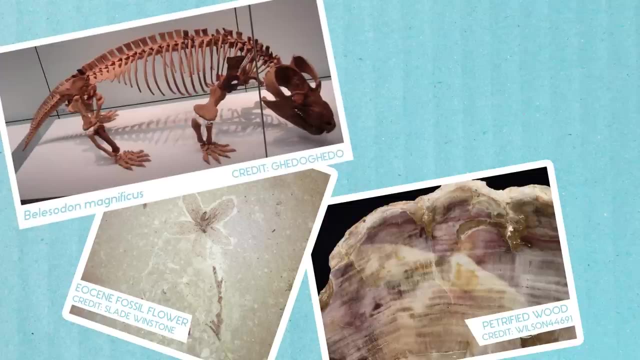 of life on Earth. For example, they've learned about extinct trees and flowers that lived millions of years ago. They found bones of some of the earliest known mammals And, of course, if it weren't for fossils, we wouldn't even know dinosaurs existed. 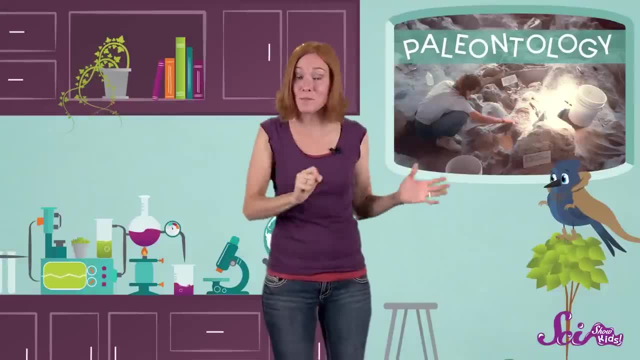 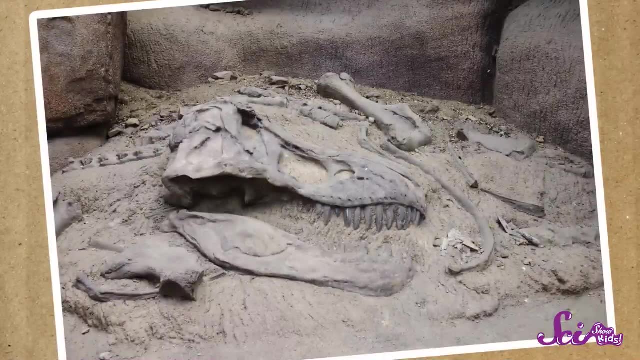 Paleontologists have been able to make all of these discoveries because they're experts at reading the clues they find in fossils. If scientists find enough bones belonging to an extinct animal, like a dinosaur, they can put them together to figure out what that animal looked like. 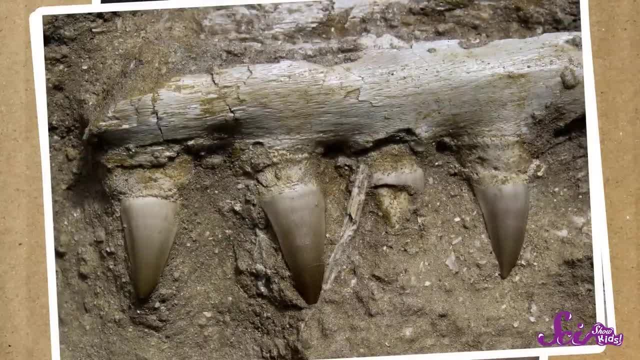 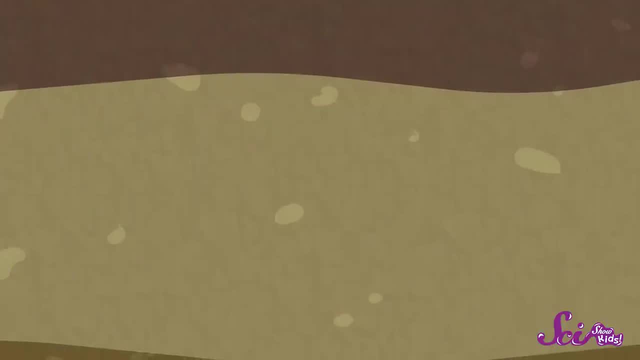 And if they find the dinosaur's teeth, they can figure out whether it ate plants or other animals or both. Just knowing where a fossil is buried can give scientists a lot of information too, For example, if paleontologists come across a layer of rock with a lot of the same kind. 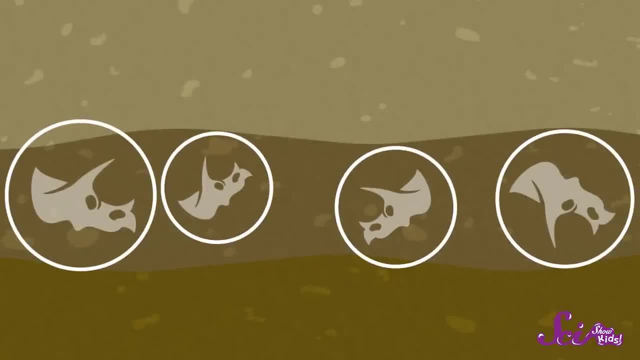 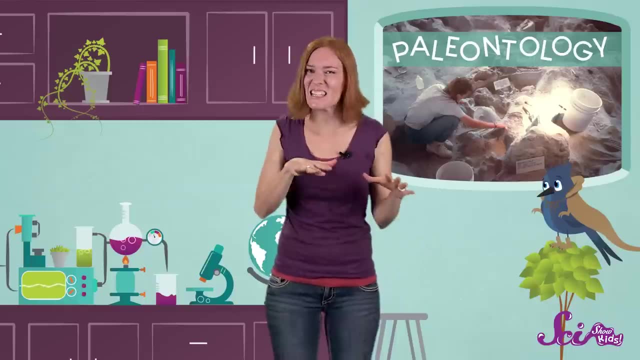 of dinosaur fossils in it. that might mean that that kind of dinosaur lived in big groups. But before paleontologists can study fossils, they have to find them first, And that means that these scientists get to spend lots of time outside digging in the 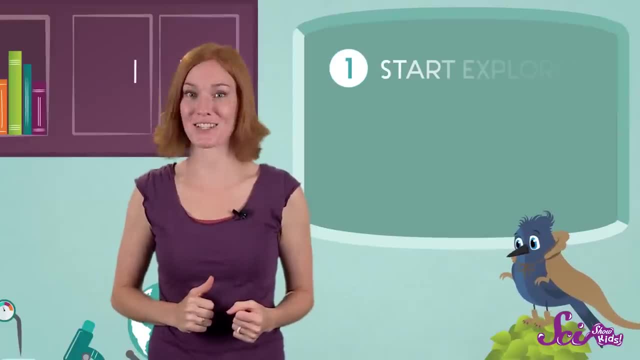 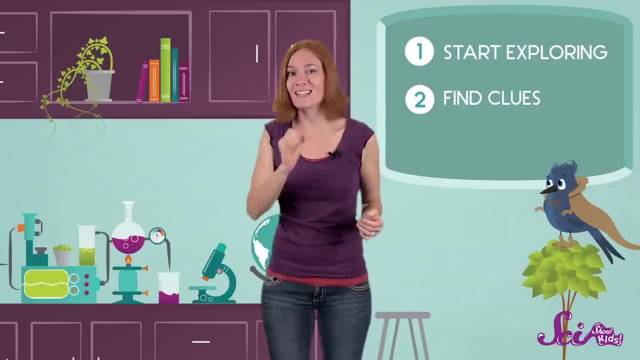 dirt. First, they go to areas where they think fossils might have formed and start exploring. They keep their eyes open for small bits of bone sticking out of the ground or rocks with cool shapes on them. Riverbeds and hillsides are especially good places to look. 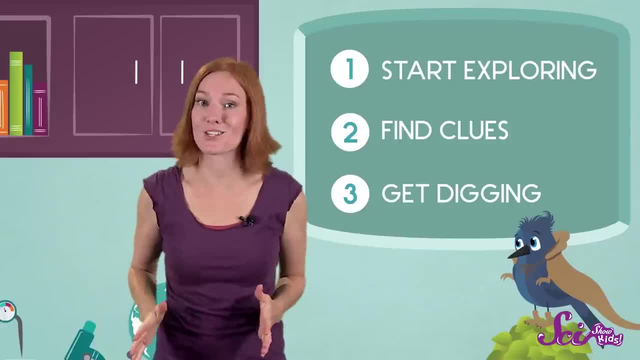 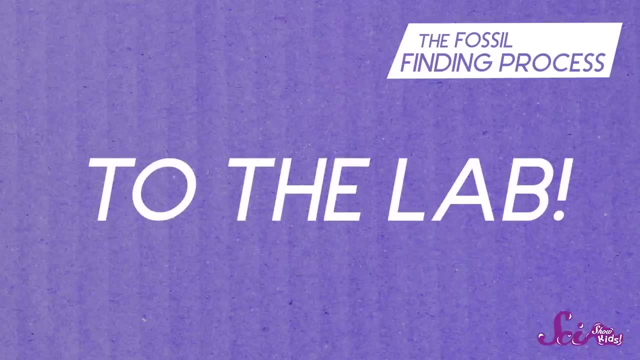 Once they find a promising spot, it's time to get digging. Paleontologists use picks, shovels, even big diggers, to unearth their finds. If they uncover a fossil, then they take it back to their laboratory to study it. 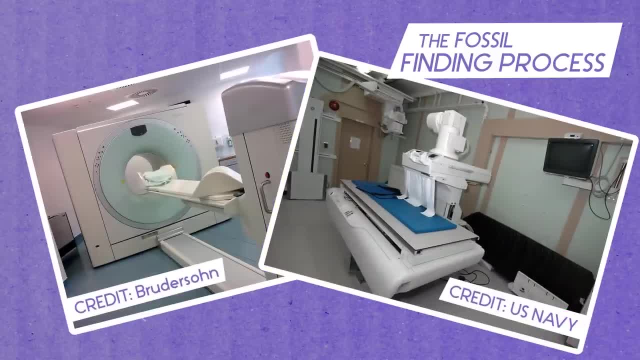 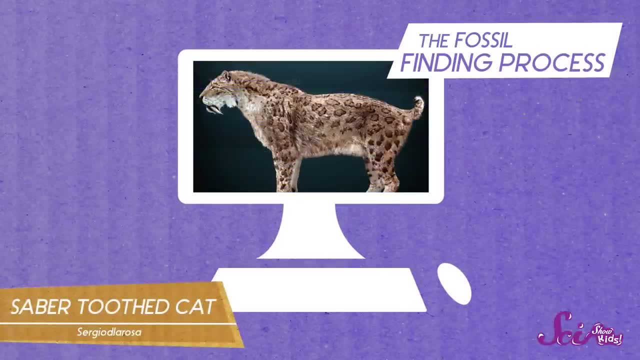 There. they can use cool technology like x-ray machines and CT scanners to see inside the fossil, And they can use computers to help them see what the plants and animals may have looked like when they were alive. And finally, paleontologists spend a lot of their time sharing their discoveries with 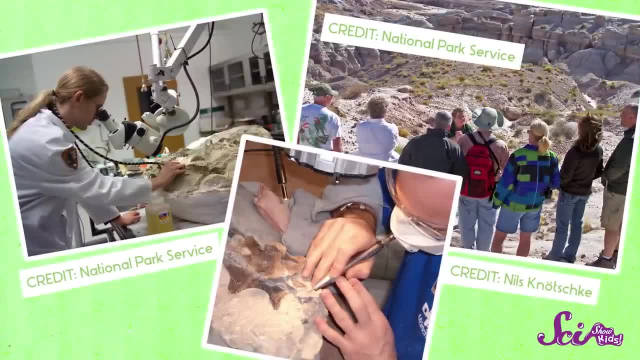 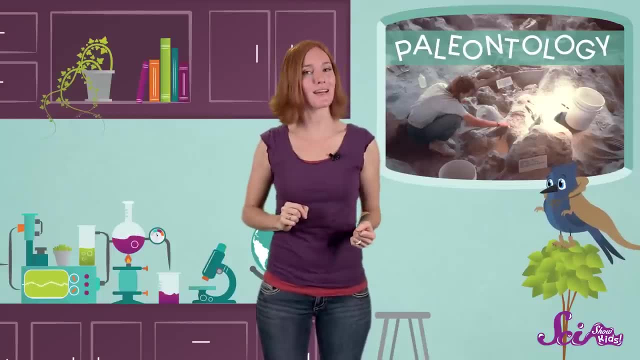 other people. Lots of paleontologists work with museums and schools so that they can teach people like you and me about fossils that they find, And the fossils are usually kept in museums or universities so other scientists can study them too. All told, digging in the dirt and dreaming of dinosaurs may look like fun, but they're.